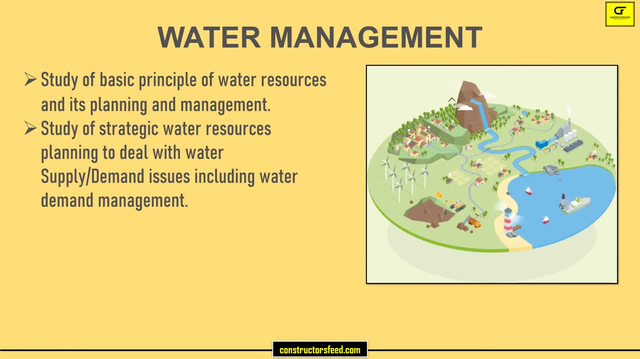 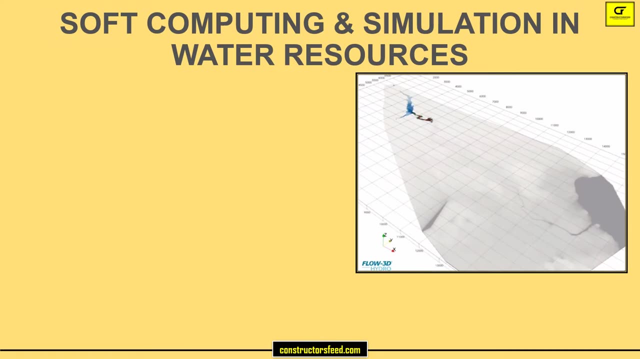 Study of strategic water resources. planning to deal with water supply slash, demand issues, including water demand management. Study of reservoir storage and other structural and non-structural methods. These are the reference books. Reference Book: Soft computing and Simulation in water resources. Study of application of the latest information technology to water sources. engineering. 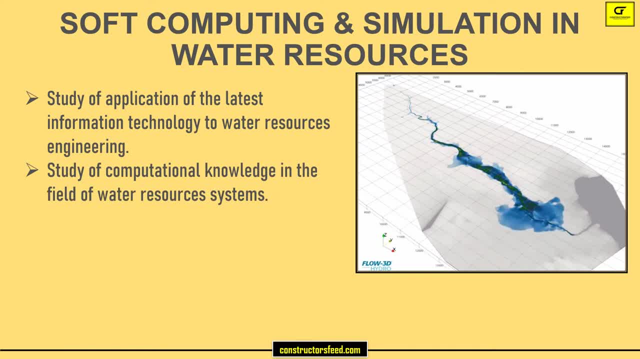 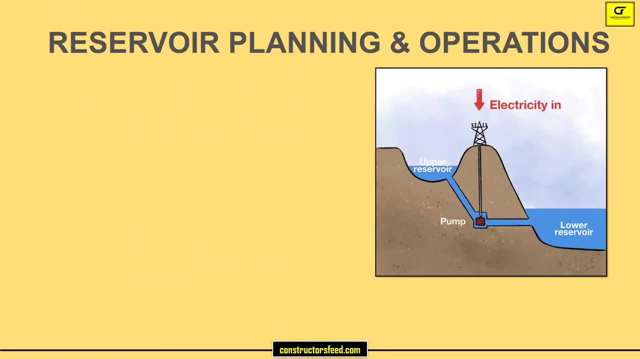 Study of computational knowledge in the field of water resources. Reference引: Study of computational knowledge in the field of water resources, of water resources systems, study of simulation models and use the latest intelligent technology and algorithms. these are the reference books: reservoir planning and operations. study of reservoir planning- multi objective. 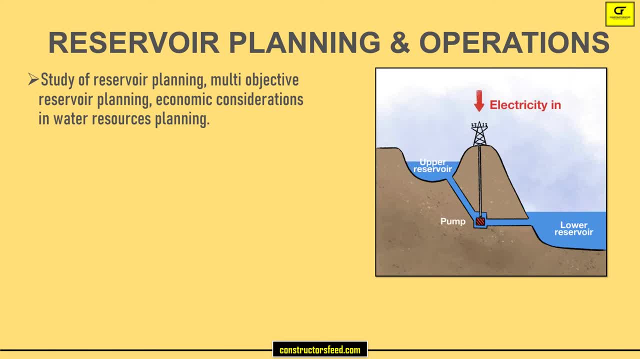 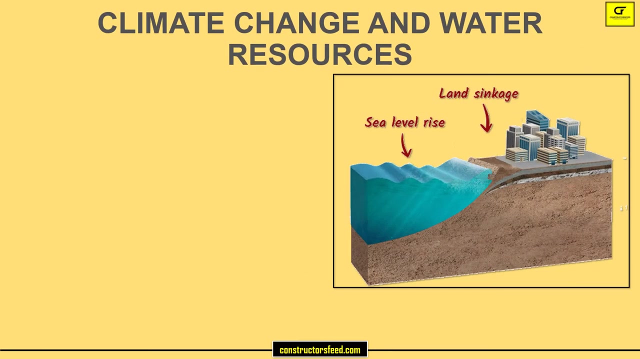 reservoir planning. economic considerations in water resources planning. study of optimal operating policies and multi reservoir systems policies. study of water quality control in river systems. study of ground and surface water and crop yield optimization. these are the reference books. climate change and water resources. study of the impact of climate change on 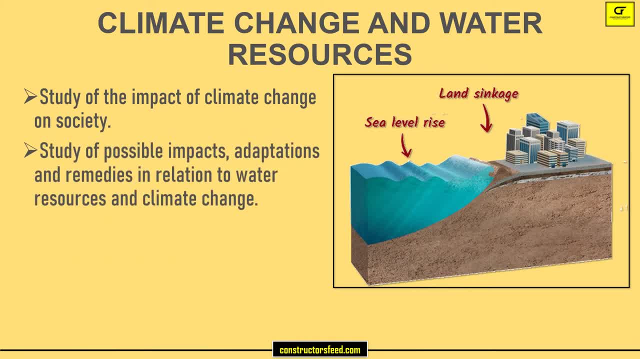 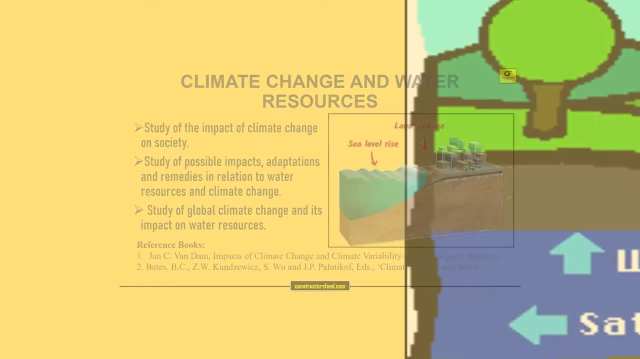 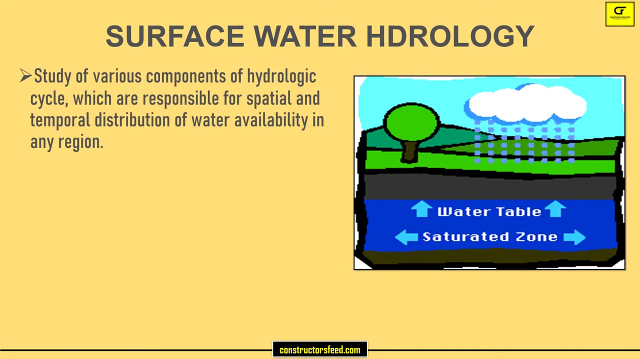 society. study of possible impacts, adaptations and remedies in relation to water resources and climate change. study of global climate change and its impact on climate change and its impact on climate change and its impact on water resources. these are the reference books. surface water hydrology. study of various components of hydrologic cycle which are responsible for spatial and 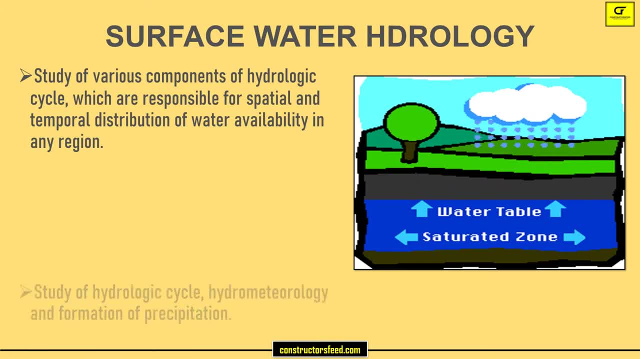 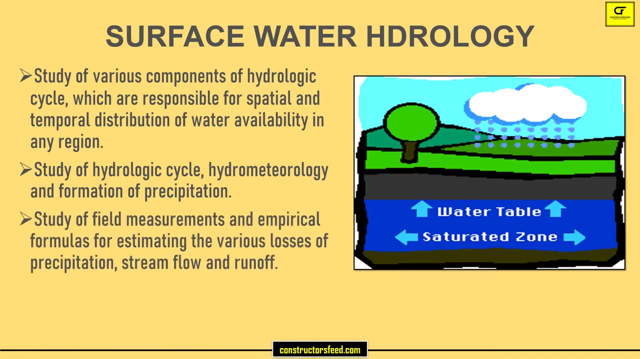 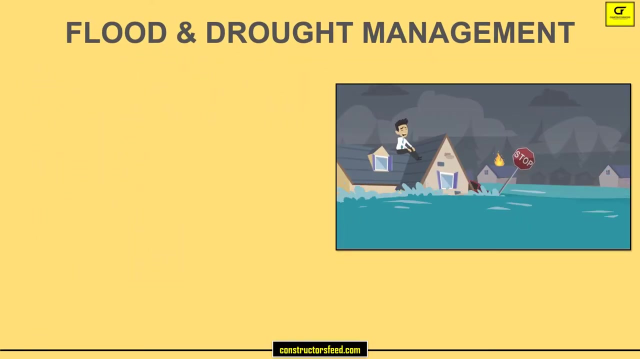 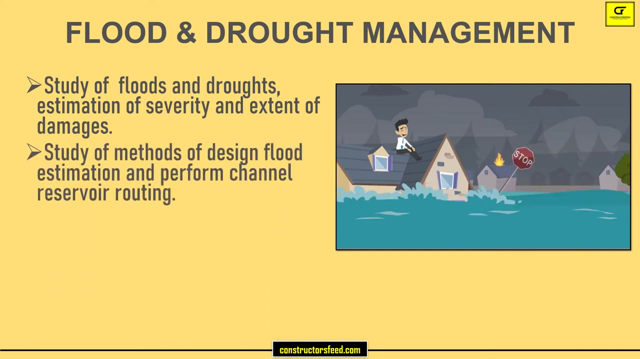 temporal distribution of water availability in any region. study of hydrologic cycle, hydro meteorology and formation of precipitation. study of field measurements and empirical formulas for estimating the various losses of precipitation and water loss. estimating the various losses of precipitation and water loss gårding Canadian cod, despite the Shepherd tributaries. and aneter. These reports are the references books. flood and drought management. study of floods and droughts, estimation of severity and extent of damages. study of methods of design, Flood Estimation and Perform Channel Reservoir rooting. study of frequency of drought using indices. these are the reference books. these are the references books. water power generation: public worry worth increasing water resource구요's standards and Sauvage direct. thank you, 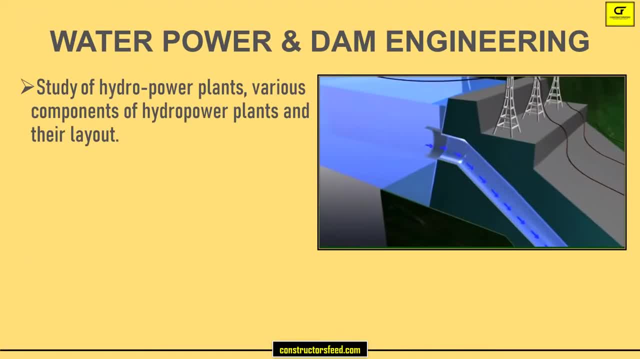 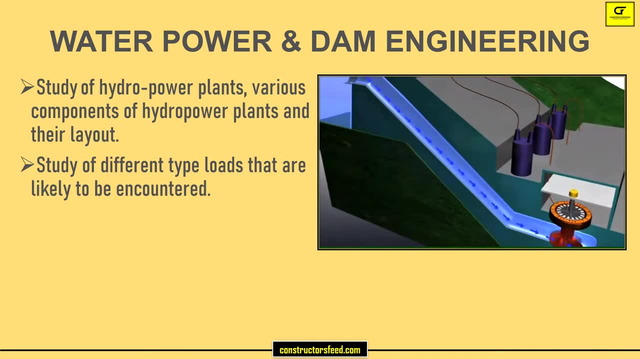 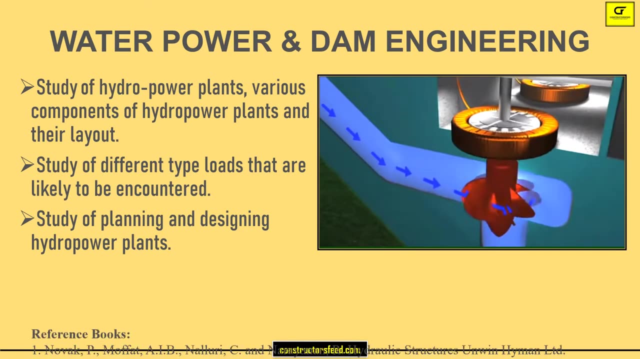 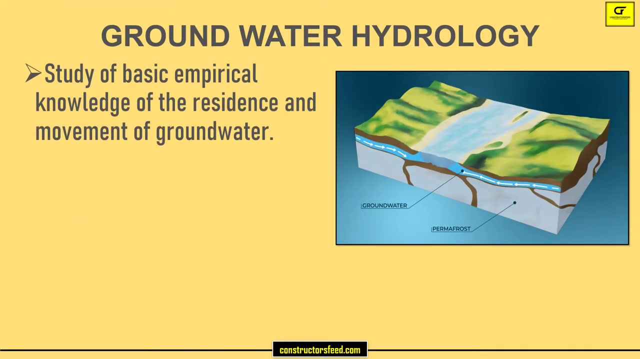 and dam engineering. study of hydro power plants. various components of hydro power plants and their layout. study of different type loads that are likely to be encountered. study of planning and designing hydro power plants. these are the reference books: groundwater hydrology. study of basic empirical knowledge of the residents and movement of groundwater. study of aquifer. 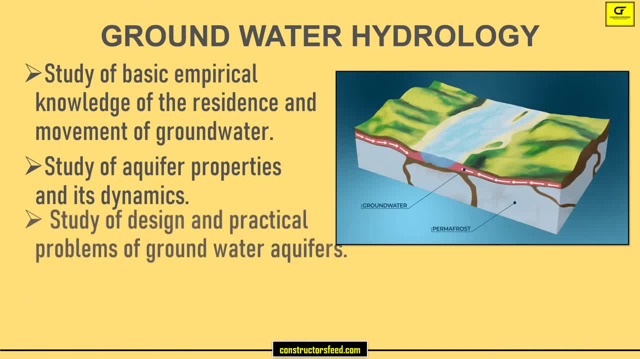 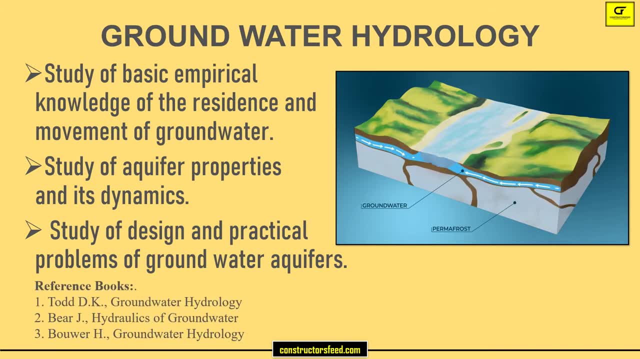 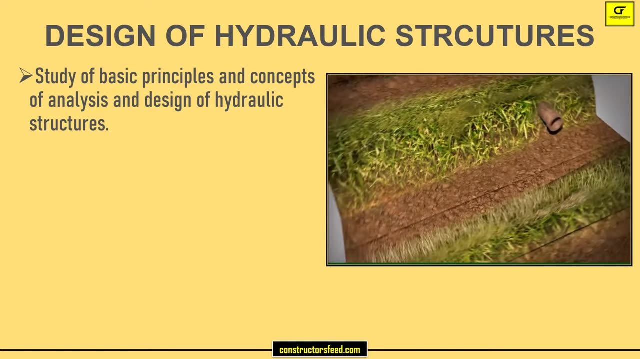 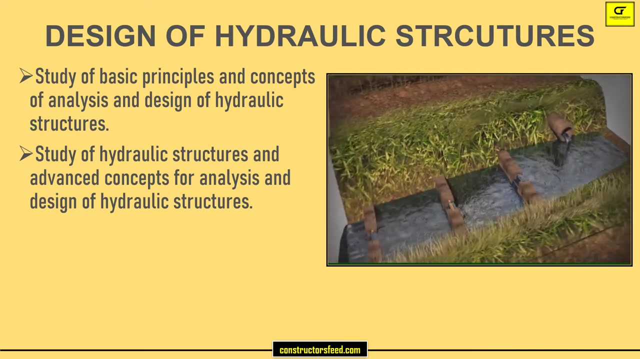 properties and its dynamics. study of design and practical problems of groundwater aquifers. these are the reference books. design of hydraulic structures. study of basic principles and concepts of analysis and design of hydraulic structures. study of hydraulic structures and advanced concepts for analysis and design of hydraulic structures. study of integrating the hydraulics. 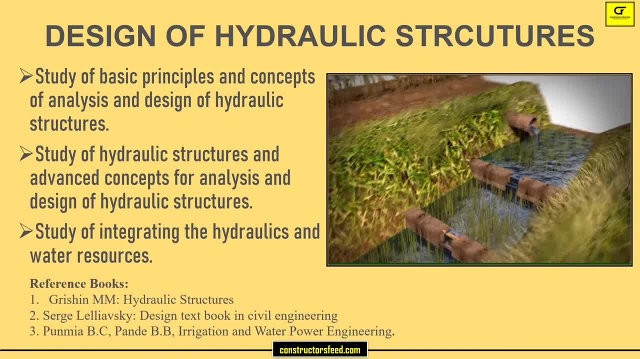 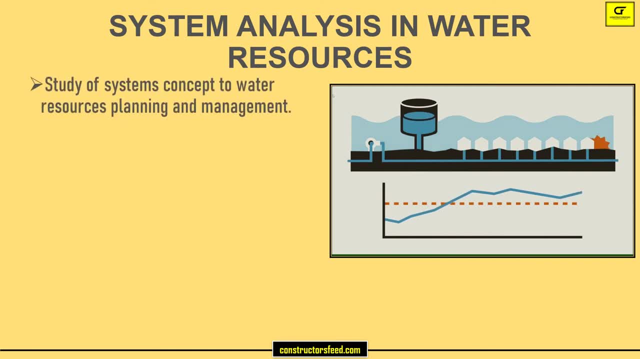 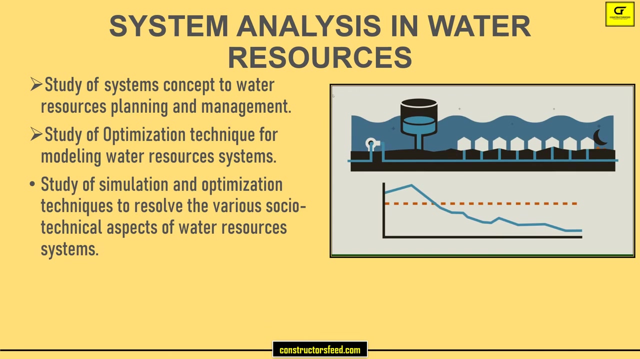 and water resources. these are the reference books: system analysis in water resources. study of systems concept to water resources planning and management. study of optimization technique for modeling water resources systems. study of simulation and optimization techniques to resolve the various socio-technical aspects of water resources systems. these are the reference books. 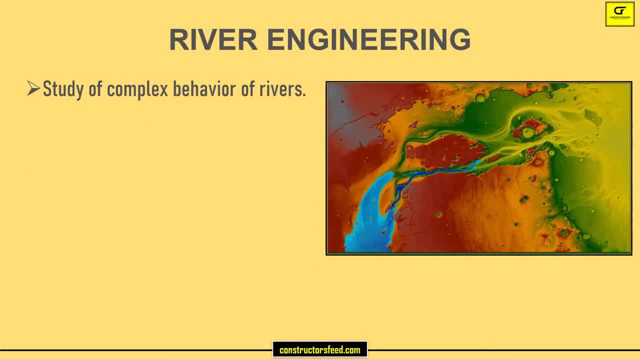 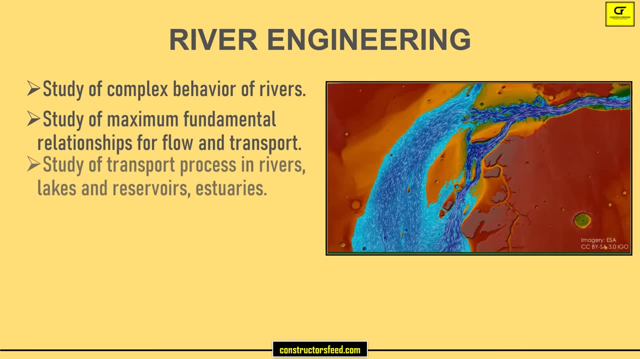 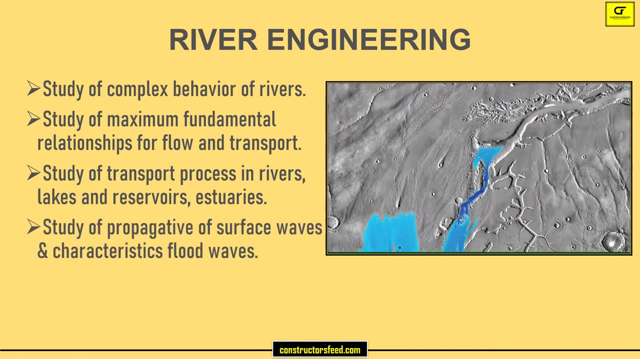 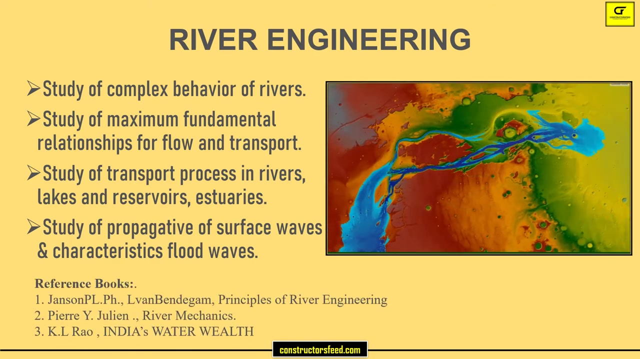 river engineering. study of complex behavior of rivers. study of maximum fundamental relationships for flow and transport. study of transport process in rivers, lakes and reservoirs, estuaries. study of propagative of surface waves and characteristics flood waves. these are the reference books. elective subjects: analysis and design of concrete dams. 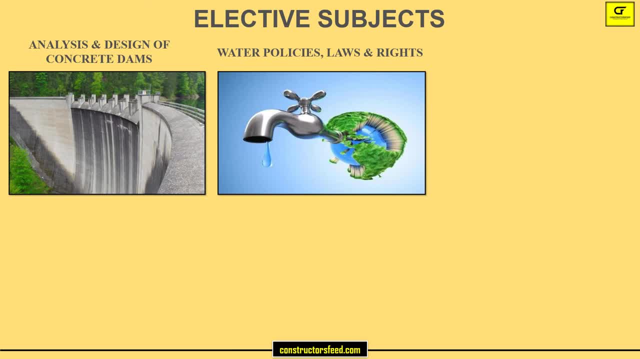 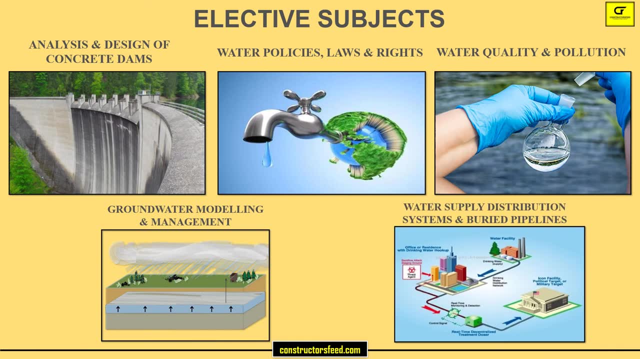 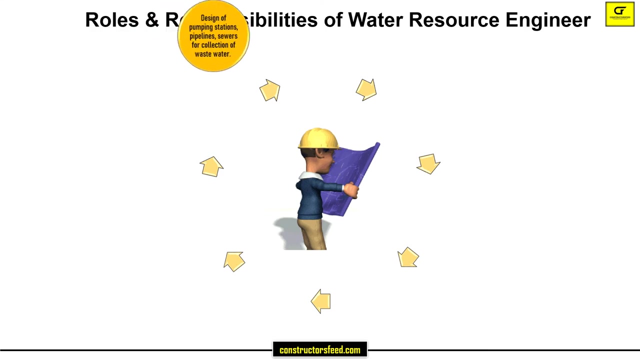 water policies, laws and rights, water quality and pollution, groundwater modeling and management, water supply distribution systems and buried pipelines. some of the roles and responsibilities of water resource engineer: design of pumping stations, pipelines, sewers for collection of wastewater, Analyzing and recommending chemical, biological treatment methods.